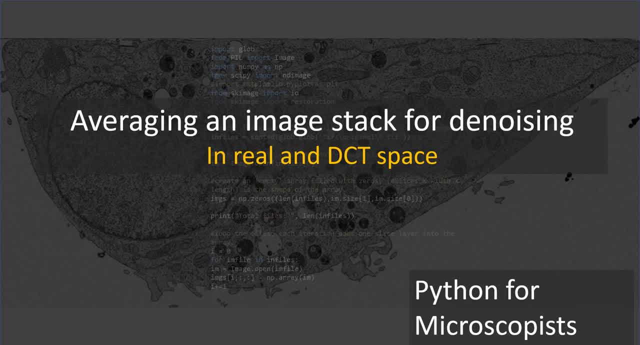 difference between DFT and DCT and because DCT contains most of the information in a small subset of these coefficients, it's highly desired in the compression type of algorithms. Now for this tutorial. let's actually do something fun. Let's perform denoising by averaging an image stack. As you probably know, if you have a stack of images, 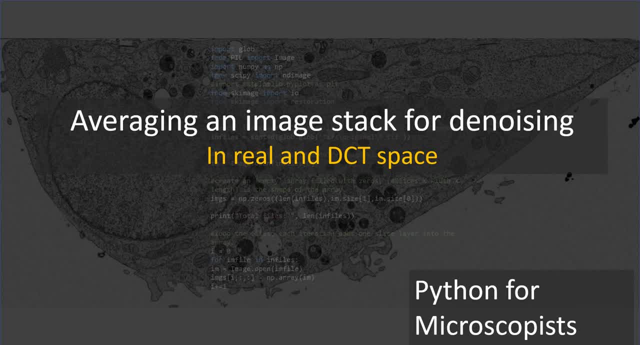 with some random noise in each image, then by averaging it, you can reduce the noise and you can get clean images. Now you can do that in real space, obviously by taking each image and averaging it, but we are also, at the same time, going to do that in the DCT space: discrete cosine transform. 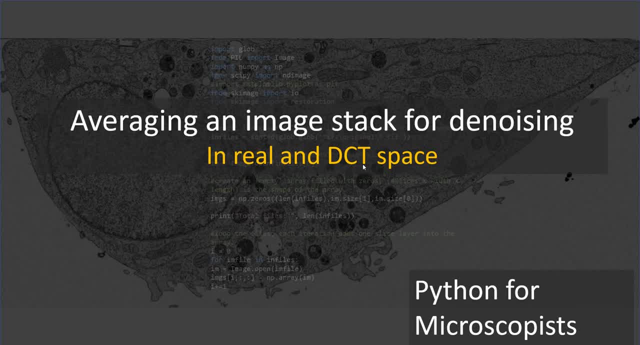 space. By the way, you can repeat this exercise on DFT space. the result will look very similar. okay, So we are going to convert each noisy image into DCT space and we are going to average all the DCT images and convert that averaged image back to the real space, and then we are going to do the same with the real 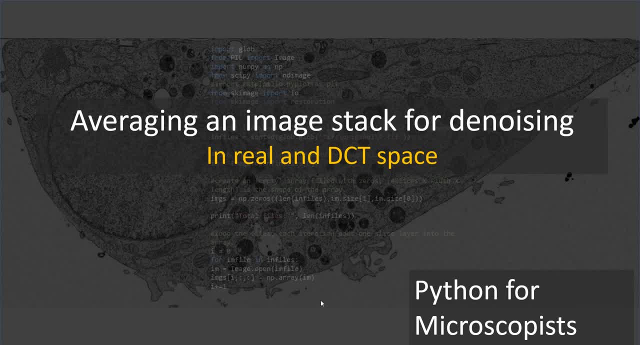 images and see how the outputs compare. Spoiler alert: DCT, just like DFT, is linear, which means you shouldn't see much of a difference whether you work on the real space or DCT space, unless you start manipulating things in DCT space and converting back to real space. So we are going to 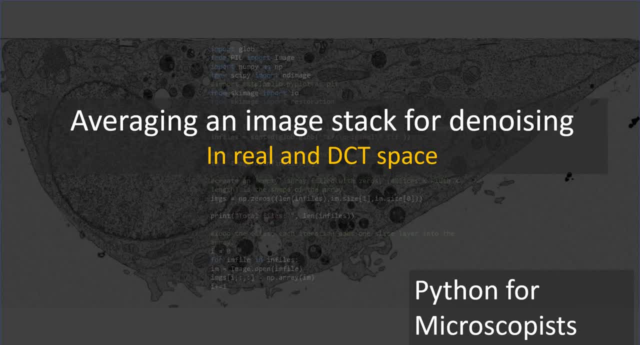 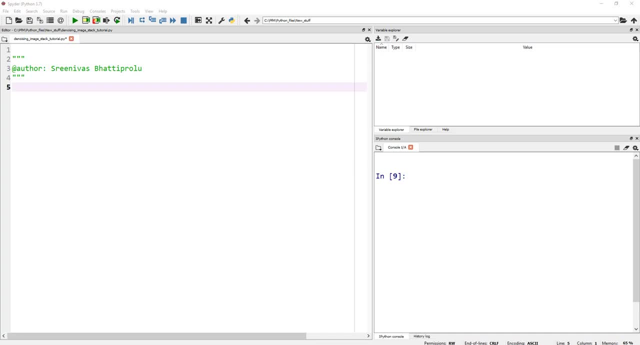 do that in the real space, just like we did in the previous tutorial. okay, So let's jump into spider IDE to code this, and I've already written parts of the code, so let me go ahead and copy chunks at a time so I can explain it. So, first of all, the headers. yeah, we always start by importing. 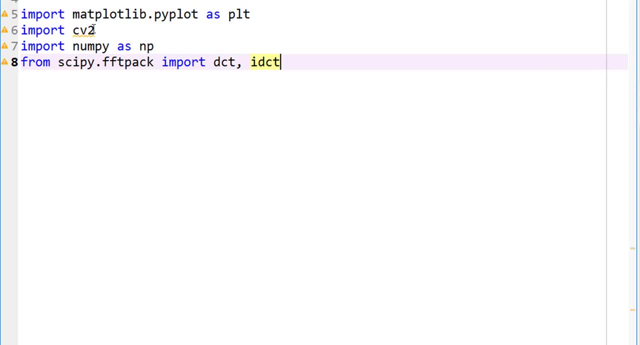 the right library. so I'm going to import the pi plot. I'm going to import cv2 so I can read images, and numpy so we can manipulate numbers, and the DCT and inverse discrete cosine transform are both available as part of FFT pack in SciPy package. okay, So this is how we are going to import them. 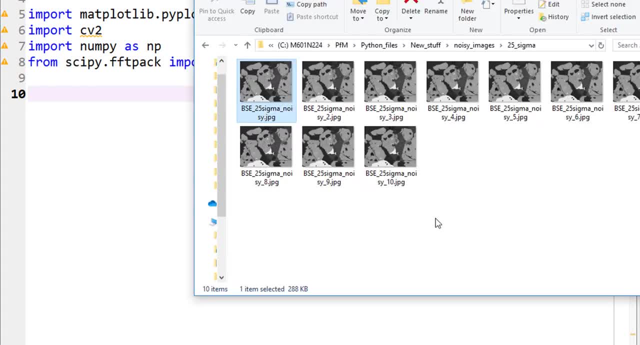 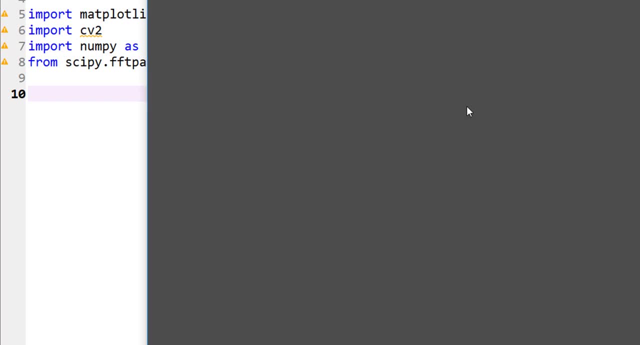 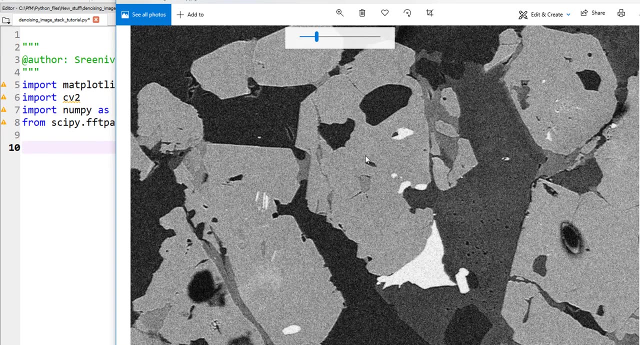 and now my images are located in a directory called 25 Sigma and I have about 10 images, and if I open the first image, you can see that this is indeed a relatively noisy image. so there is some noise right there, and let's actually average all the images to hopefully denoise these. Now how? 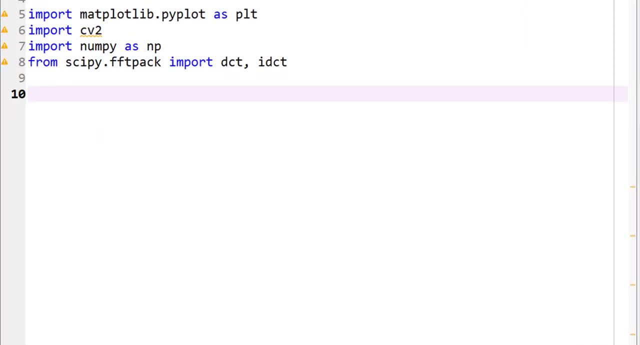 do we read a whole bunch of images? Well, there are many different ways to read images. There are many ways to read in images and for now let's actually use list directory. So I am assigning a variable called image directory and then obviously to define my directory there and the next step is to 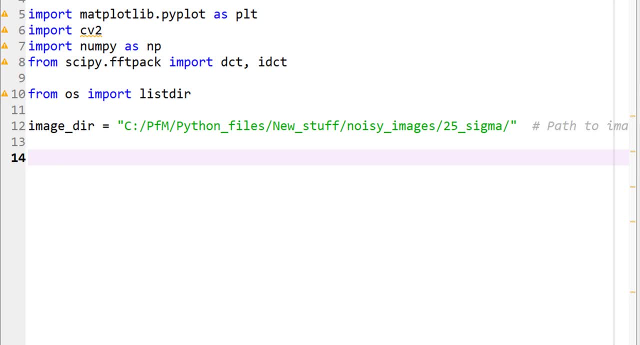 load the images. okay, So let's load images one at a time. so right there. so we are going to load the images. okay, So for F in file name, so it's going to actually go through each file within that folder and then we are going to use cv2.imri to read these and I'm reading each image as a gray scale image. 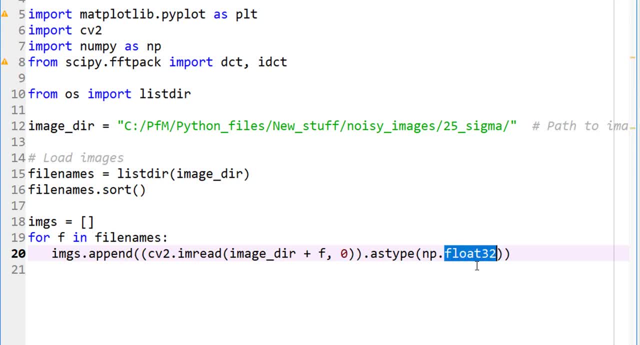 and I'm reading each image as float 32.. So for any of these operations, whether it is DFT or DCT, they like to work with floating point 32 numbers. okay, That's the reason I'm converting them into floating point 32.. Now the next thing is we need to average these images right. So to average the images first. 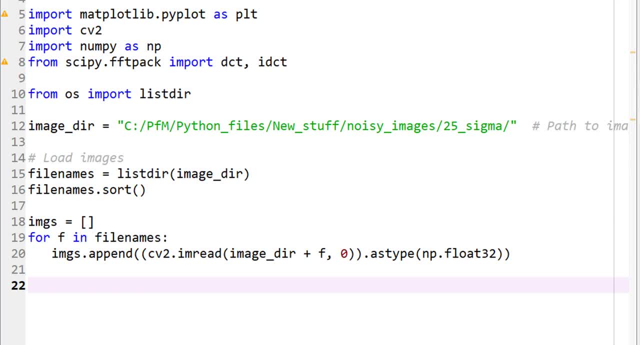 of all, let's define placeholders to actually store the images. So let's define placeholders to actually dump our numbers, the averaged numbers, into. So I'm going to define a couple of placeholder placeholder arrays. So first of all, I'm reading the images and I'm extracting what the height and 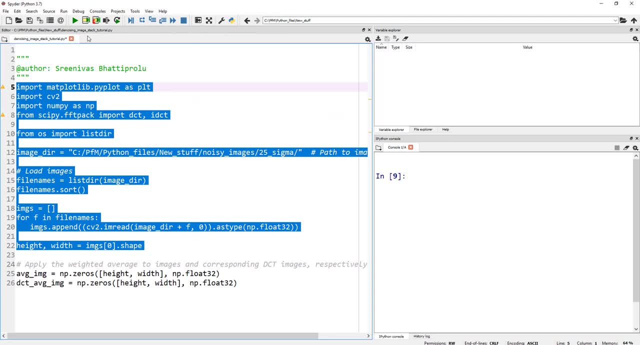 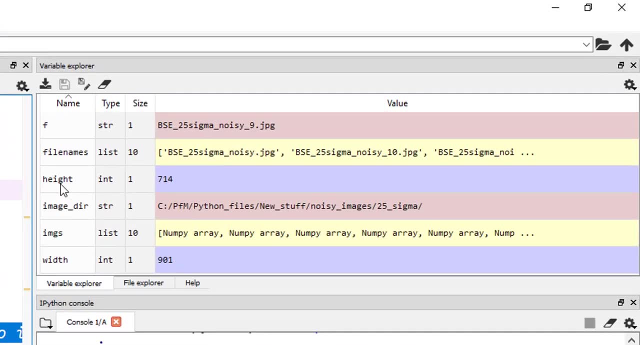 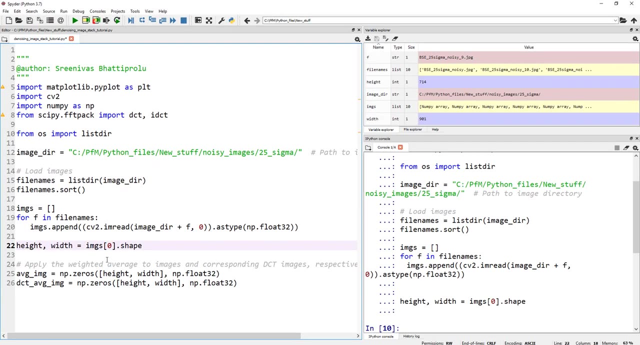 width of these images are okay. So first let's actually run the code until this point, okay, So you can see what I'm looking at here. So my images have a height of 714 and width of 901.. So my height here is 714, width is 901. okay, And just to give you a little bit of a sense of what I'm looking at. 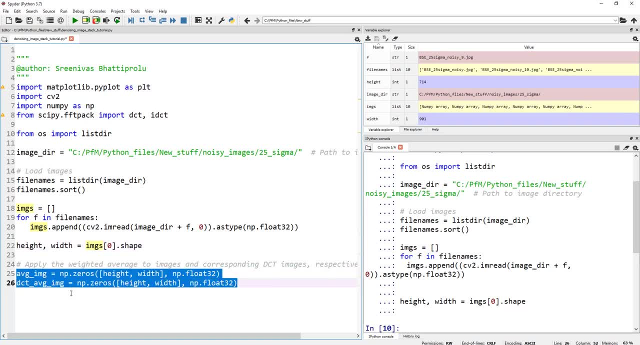 here. So my images have a height of 714 and width of 901.. So my height here is 714, width is 901. okay, And then I'm creating empty. So let's actually run this part of the code: Average image, AVG image up. 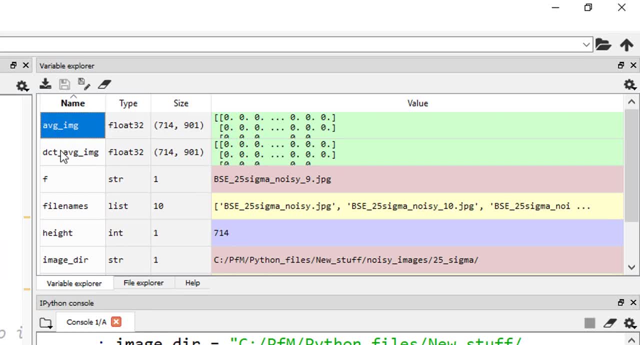 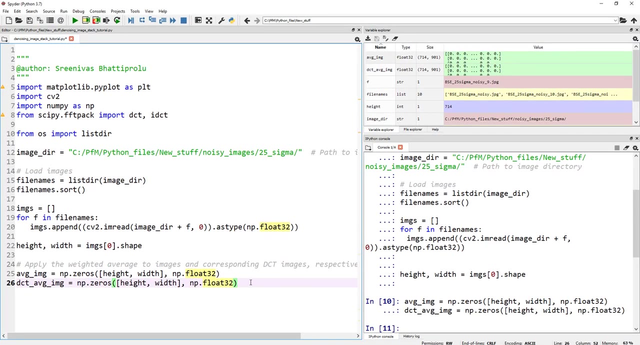 there. As you can see, I'm creating two empty arrays, numpy arrays of float 32 type- yeah, of float 32 type, And the size of this array is 714 by 901, and they're filled with bunch of zeros, for now, okay, Later on we'll fill them with our average values, And now we just need to calculate. read each. 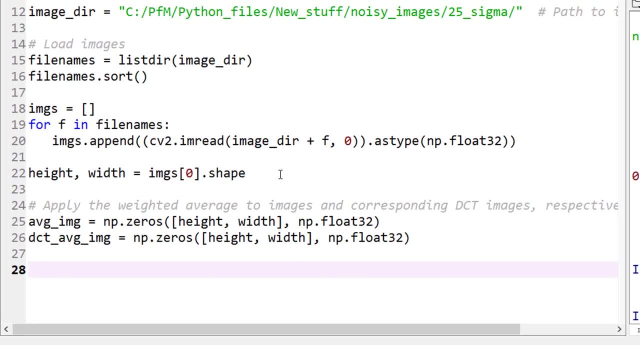 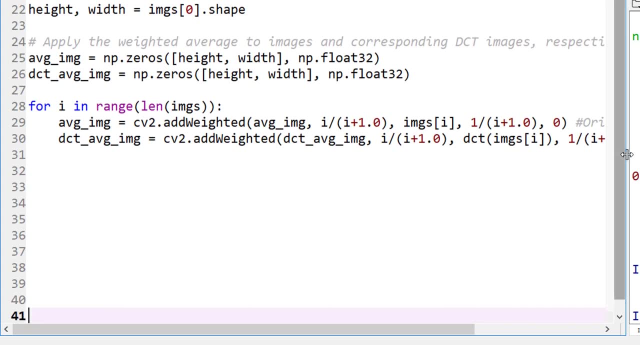 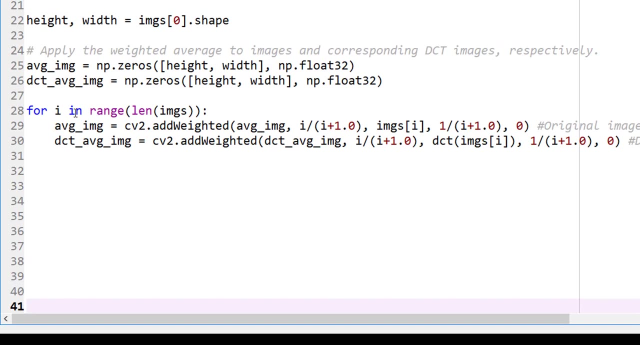 image and at every pixel we have to get the average. yeah, We have to. the way you can do that is for let me create a bit more room So you can see exactly what's going on here. okay, So for I in range, length of images, meaning, for time, each image in my out of my 10 images. okay, My averaged image. 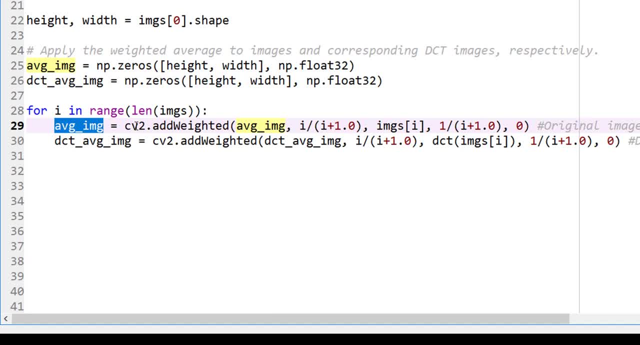 is a weighted average again. in cv2 or OpenCV There is a function called add weighted. okay, We are actually averaging the image and we are weighting it again. do the math on paper. this absolutely makes sense if you do the math, okay. So this is just a weighted average and I'm dumping. 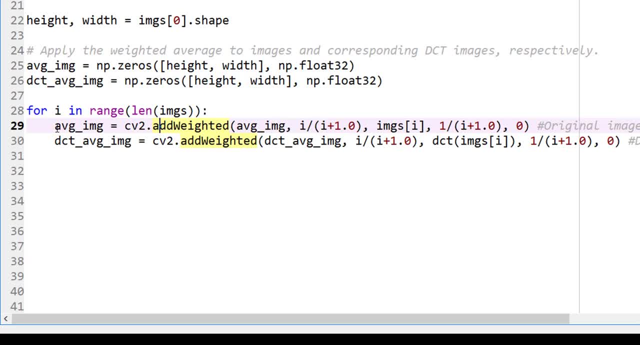 all of those values as we are going through each image into an array called average image, which we just created with with a bunch of zeros. okay, I'm doing exactly the same with my DCT, except for, instead of original images, I'm actually dumping the values of DCT of original images. 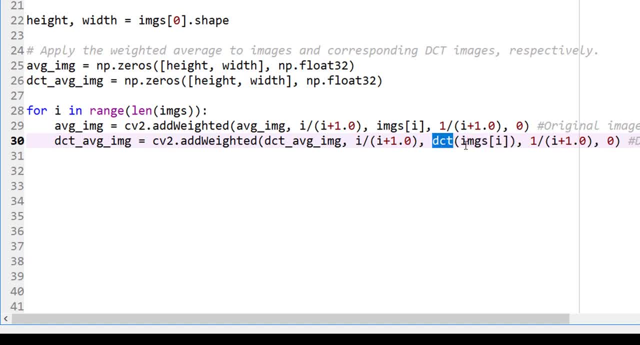 So it's actually performing DCT- discrete cosine transformation of each image- and, at every pixel, performing average and dumping that into this array. That's all it is. Now that we have our averaged DCT, let's actually get our original image back. 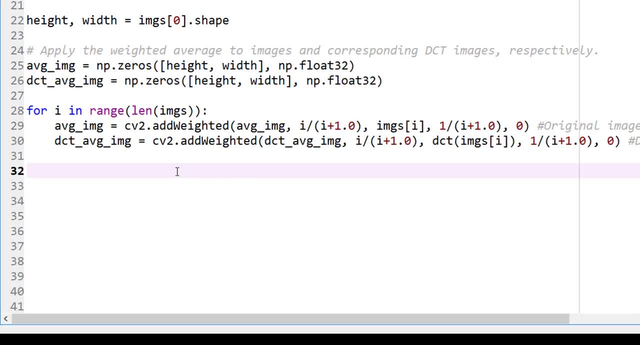 How do we get our original image back? As you can imagine, inverse DCT. So we're going to just do IDCT of our DCT averaged image. That's it. So once we have this, we just need to go ahead and have a look at these images. 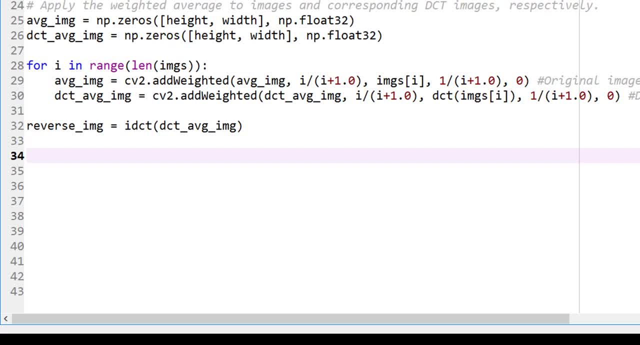 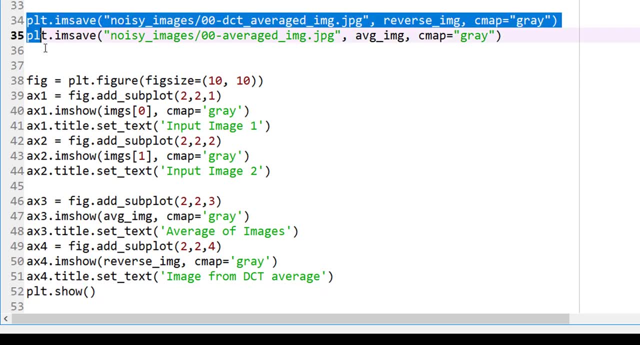 That's it. That's as simple. Now we may as well save these images. So I have written a few lines to save the images and also to look at these images on the screen. So these two lines, obviously I'm saving them by giving some appropriate names. 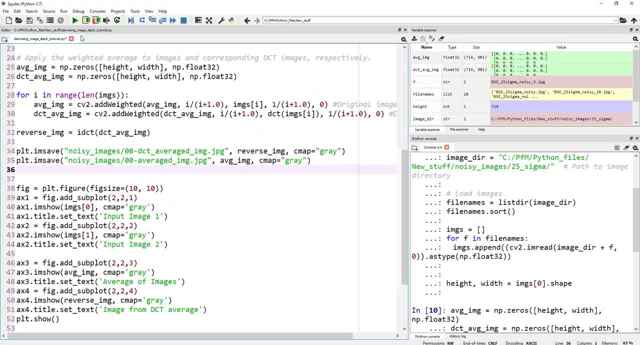 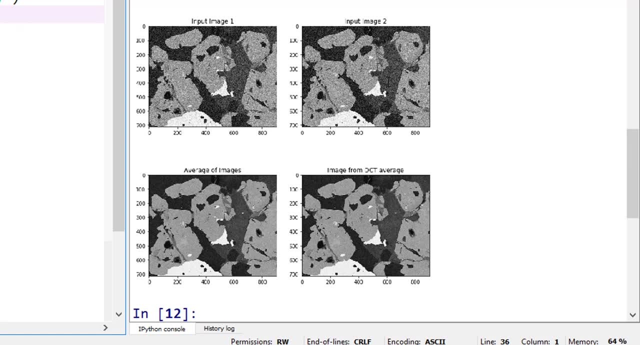 And down here we are going to visualize these images on screen. So let me go ahead and run this entire code And on the right-hand side we should see four images. The first two are the first two images, so image number one and image number two. 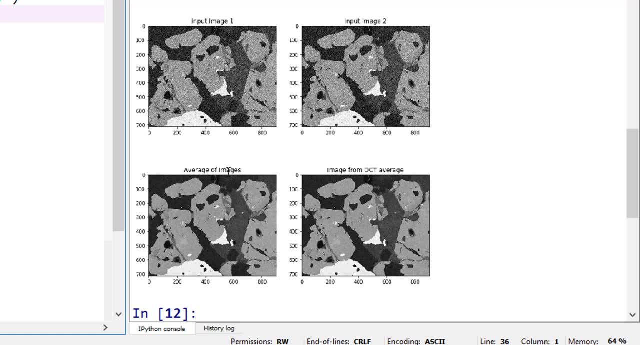 And the bottom two on the left-hand side average of images. So this is an image that we obtained by averaging all the images in the image domain And on the right-hand side is the image that we obtained by averaging all the images in. 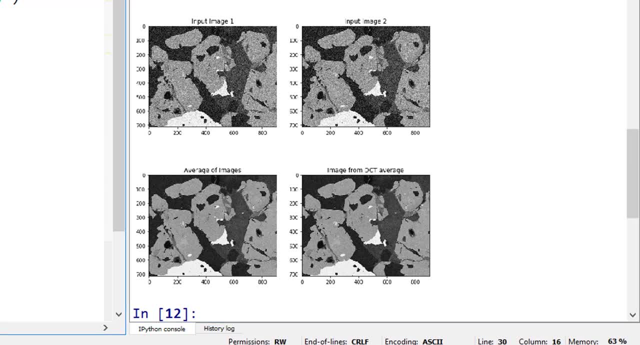 the DCT domain and then retrieving it back as images. So this is the original image. I hope I'm not confusing you guys here. As you can see, they both look very similar. In fact, if I go, and where am I saving them? 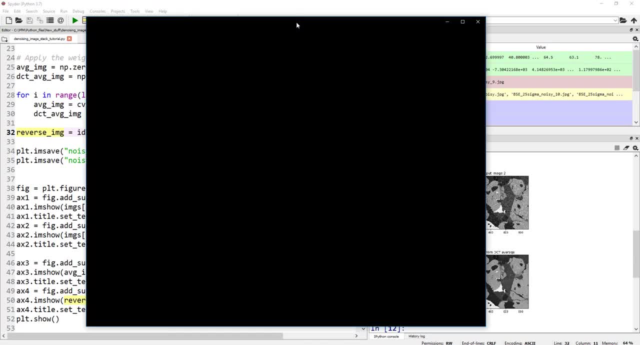 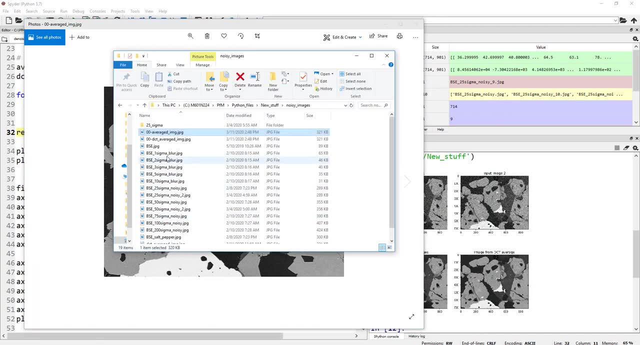 Looks like I'm saving them here. Averaged image and DCT image. they should look pretty much the same. In fact, the number should also be well not identical, but comparable. So let's actually look at these two images by putting them side by side. 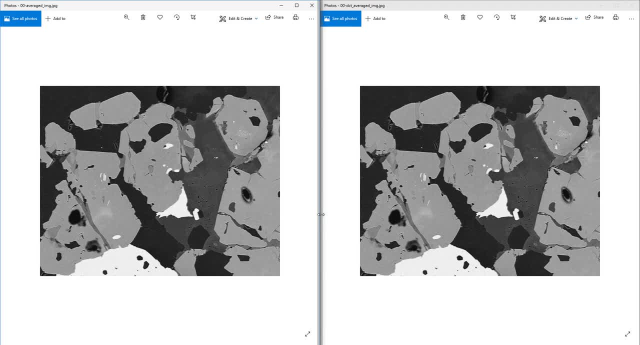 What is the best way? I think this is the best way- to put these images side by side. Okay, there you go. So don't they look identical? The one on the left is obtained by averaging pixel values of all the 10 images. okay, at. 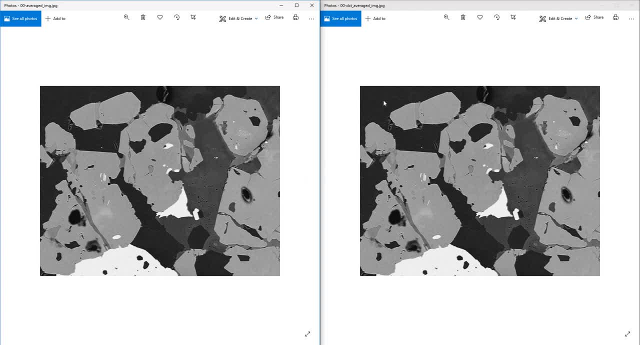 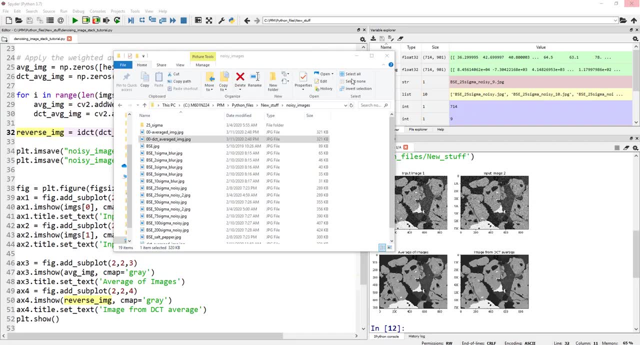 a given pixel And the one on the right-hand side is by averaging all the DCT images and retrieving the image back, They should look identical. okay, In fact, a fun exercise. in case you are curious, Go ahead and look at the average image numbers. 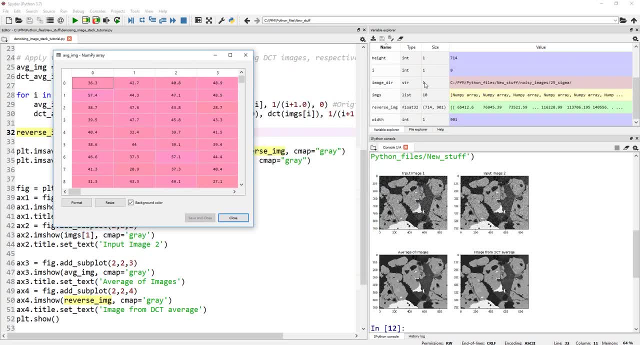 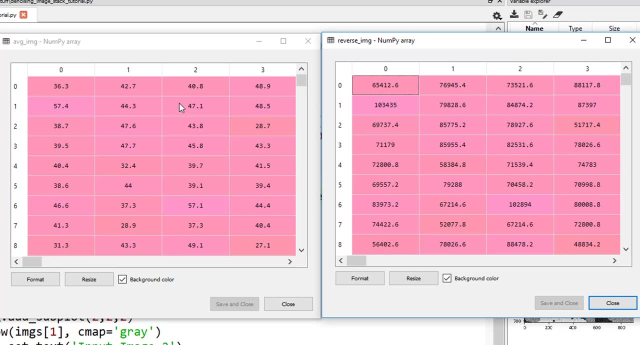 Here they are supposed to be floating point, And also look at where is our reverse image Right there. Look at these numbers. Of course they are not identical, But if you look at the scaling factor here, okay, divide 65412 by 36.3, and then take. 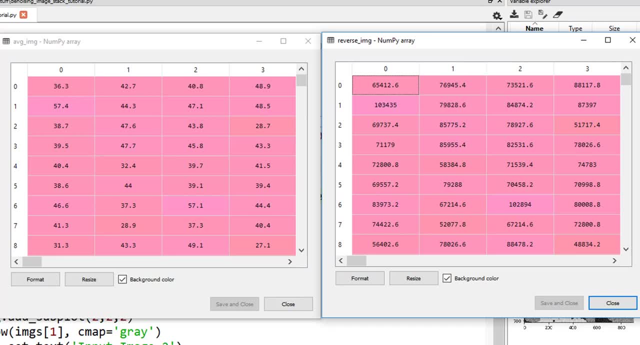 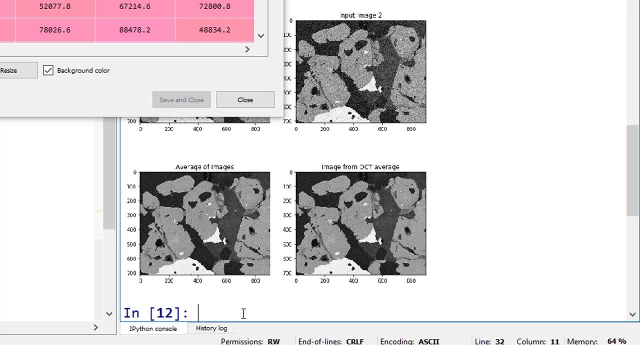 that scaling factor and you should get other numbers back. In fact, if you want me to do this, let's actually go ahead and do this exercise here, okay? So what is it? So 65412, 65412.6 divided by 36.3, 36.3 is 1802.. 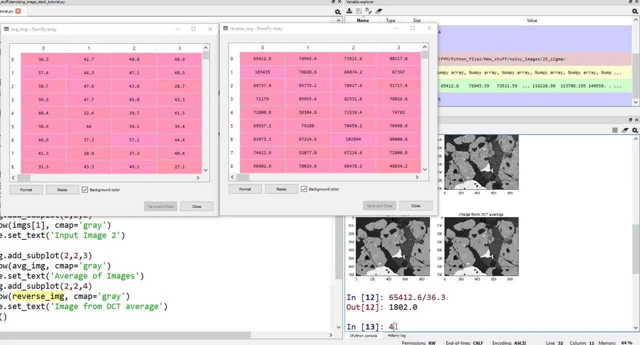 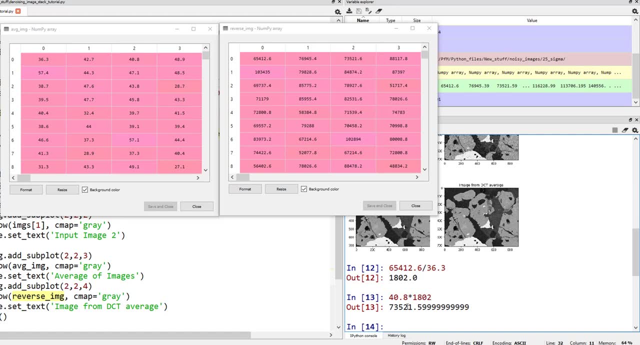 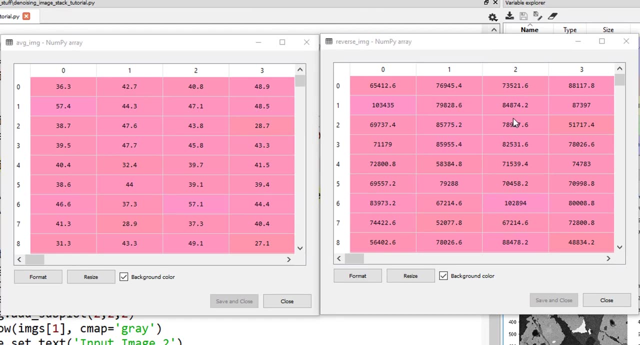 So what do we get if we multiply 40.8, 40.8 multiplied by 1802? We get 73521.5999, which is 6, right there, 73521.6.. As you can see, these two. 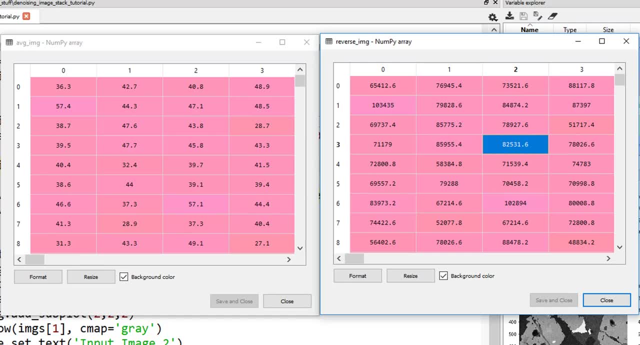 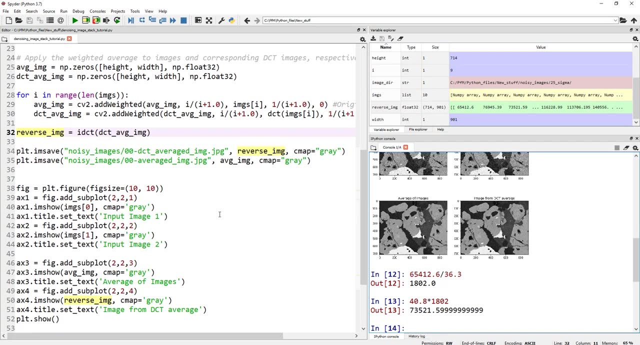 Are identical, except for the scaling factor of 1802.. So what have we proven here? What did we prove here? Well, you can do any math in the real space, convert it into, or you can do any operations in this real space, like, for example, in this case, averaging, and then convert them to. 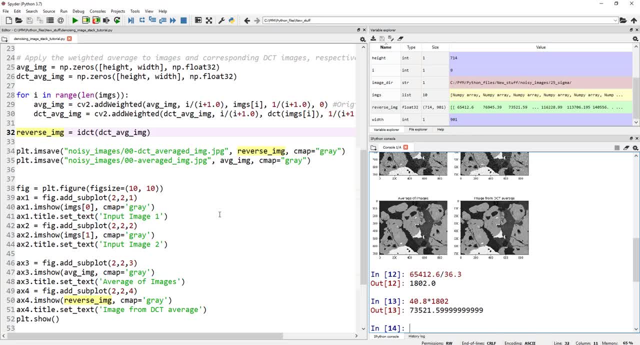 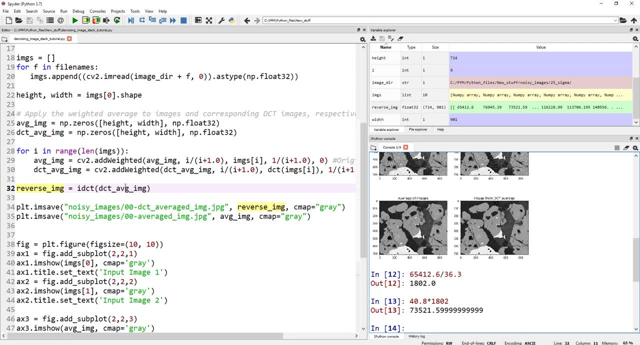 DCT, you know, and then do the average and retrieve it back. It's pretty much the same information. Now the fun lies when you actually take this DCT converted image And apply some sort of a nonlinear type of application. 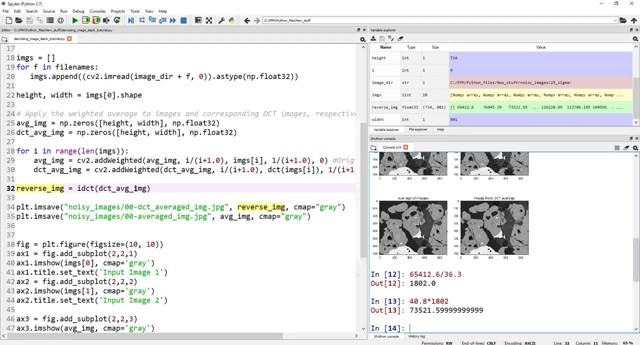 For example, blocking all the, for example, low frequency components and only letting the high frequency components. yeah, I let you do that exercise because I've done that in the previous tutorial. So do exactly the same thing using the DCT and see if you can learn something from this. 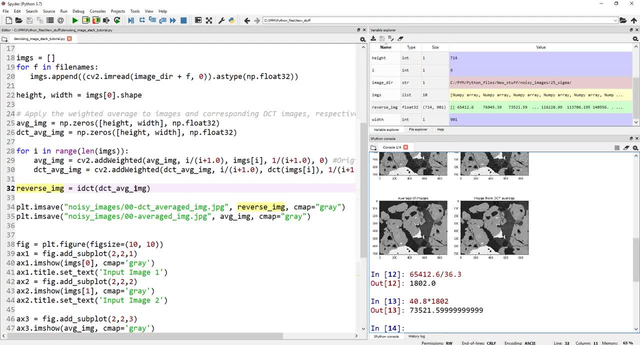 Anyway, thank you very much for your attention And if you like these type of content and this type of tutorials, please, of course, subscribe to my channel and like this tutorial on YouTube. Thank you, It always encourages me whenever I see your likes and subscriptions. 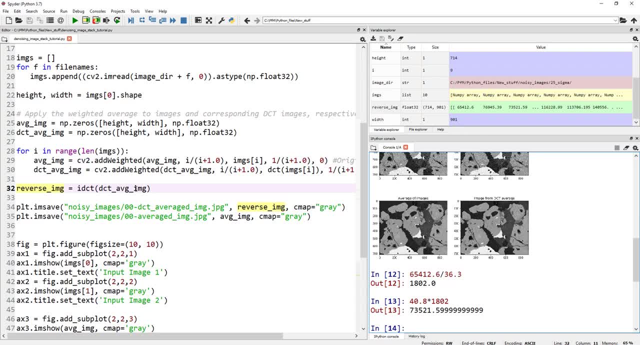 So thank you very much for your attention, And in the next tutorial let's cover a different image processing topic. 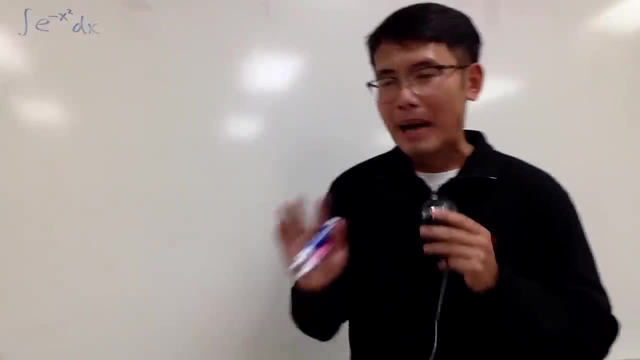 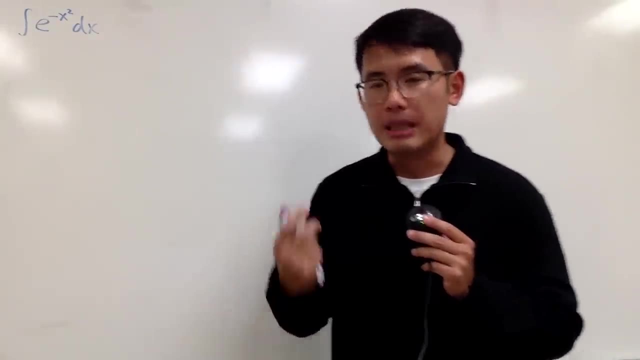 Okay, in this video we are going to integrate e to the negative x squared, But I'm not going to tell you guys to pause the video and try it first, because, no matter what you do, you cannot find an answer to this integral by using elementary functions. 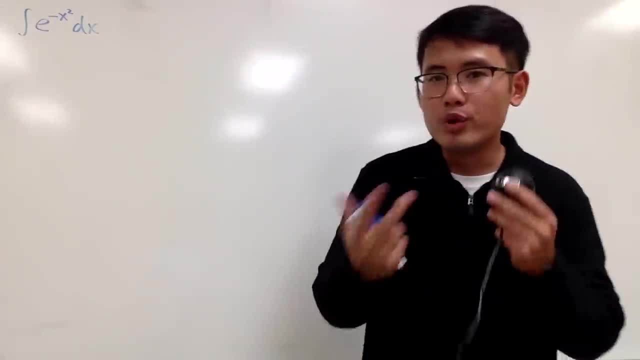 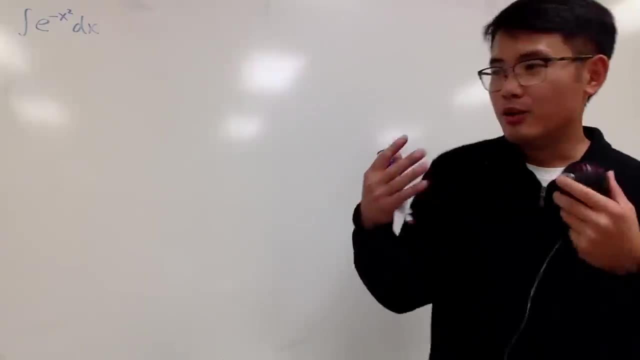 What I mean by that is, you cannot find an answer to this integral by using your regular trig functions or inverse trig functions, hyperbolic trig functions or exponential functions, logarithmic functions, radical functions, power functions whatsoever or any of the combination above.